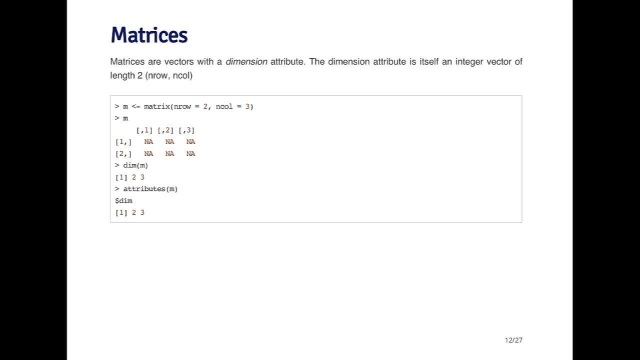 integer vector of length two, where the first number is the number of rows in the matrix and the second number is the number of columns. And so if I can create a matrix, an empty matrix, with the matrix function and I can explicitly say that, 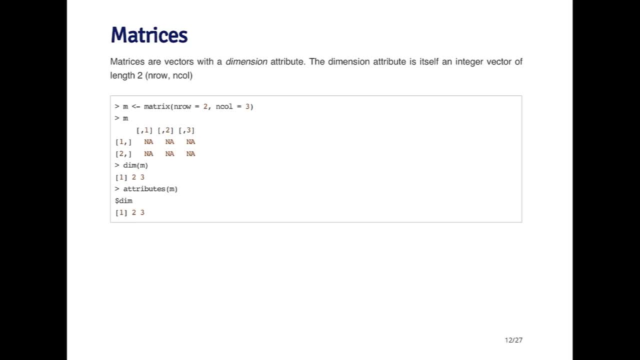 I can explicitly say how many rows and how many columns there are. This is not the only way to create a matrix, but it's one way, And so when I auto print the matrix by typing the, the object m and hitting enter, you'll see that it'll show me that. 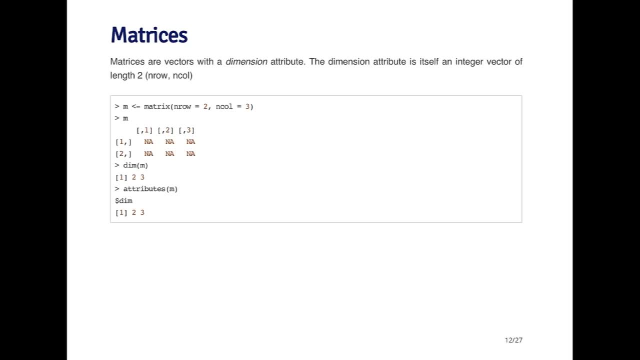 first of all, the matrix is full, is initialized with na values. There's no values in here And you can see that there's two rows and three columns and they're labeled by the numbers in the brackets. If I call the dim function on m: 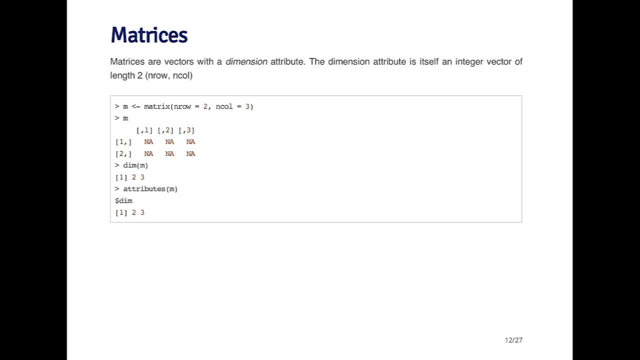 it'll give me the dimension attribute, which, in this case, it says there are two rows and three columns, because the first row is a number and the second row is a number of rows and the second number. sorry, excuse me, the first number is the. 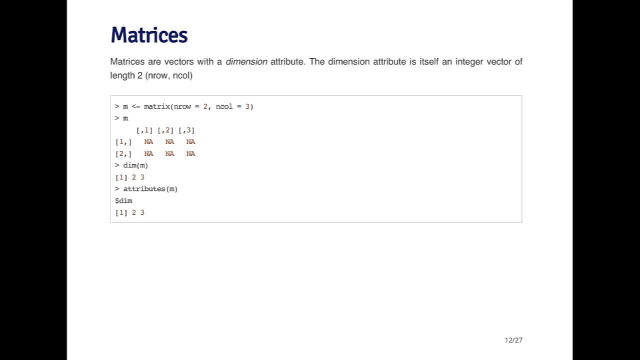 number of rows and the second number is the number of columns. If I call the attributes function on m, you'll see it returns a list where the first element is the dim element and it has the vector two, three. So these are all aspects of a. 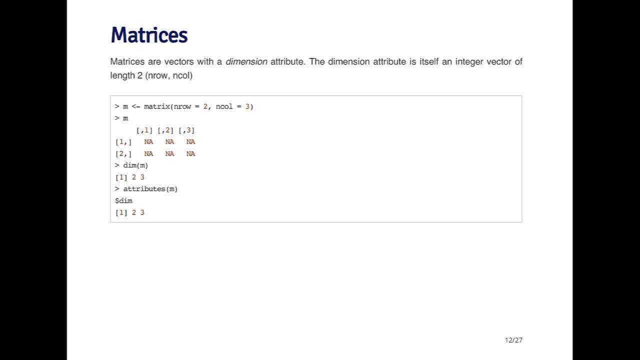 matrix, which is a vector that has a dimension attribute to it. Matrices are constructed column-wise, so you can think of the matrix taking a vector and all the numbers are inserted into the matrix by the by columns. So the first column. 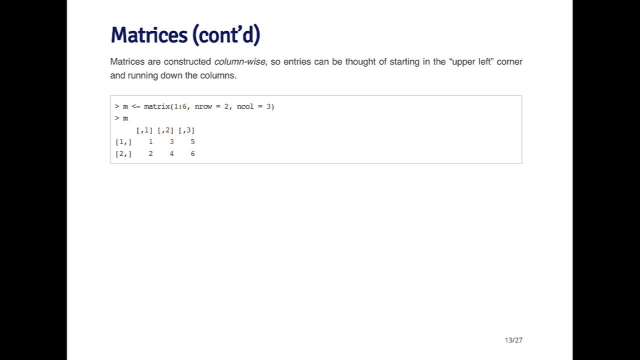 gets filled and then when the- when you hit the number- maximum number of rows- then the second column gets filled and the third column, etc. So if I create a matrix by taking the sequence one to six and then I say I specify that it has two, 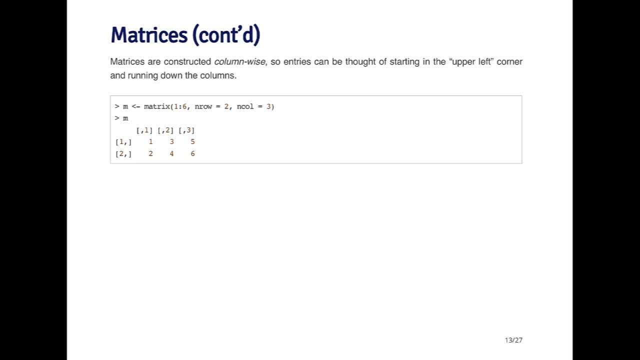 rows and three columns. well, how does this matrix get constructed? So the way it gets constructed, column-wise, so the first thing that happens is it takes one, two, and now there's only two rows, so it can only go to two, and then that makes the 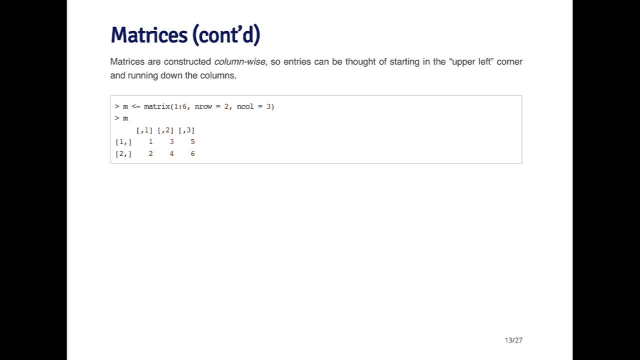 first column, The second column is made up of three, four and then the third column is made up of five and six. You can also create a matrix by creating the dimension attribute on a vector. So, for example, I can take: I can create a vector that's a. 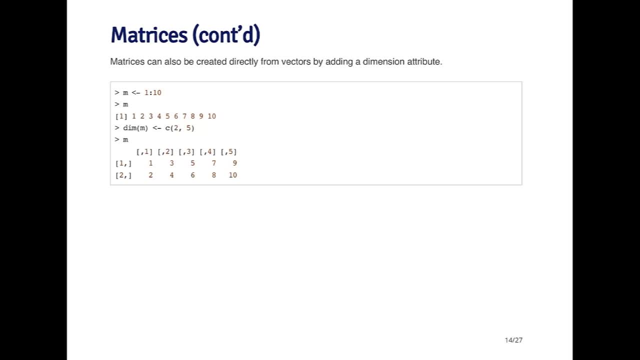 sequence one to ten, and then add the dimension attribute to it. So here I'm using the dim function, but I'm assigning a value to the dim attribute of m. So here I'm assigning the value to the dim function. So what I'm saying is: I want, I want to take this vector and transform it into a.